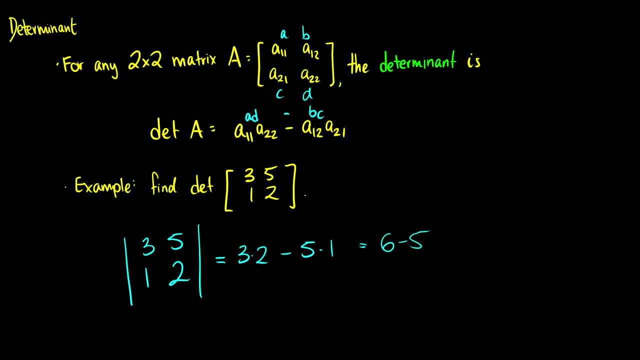 1. So this is going to be 6 minus 5, which is equal to 1.. So the determinant of this matrix is equal to 1.. And because that's not equal to 0, we know this matrix is invertible. So again. 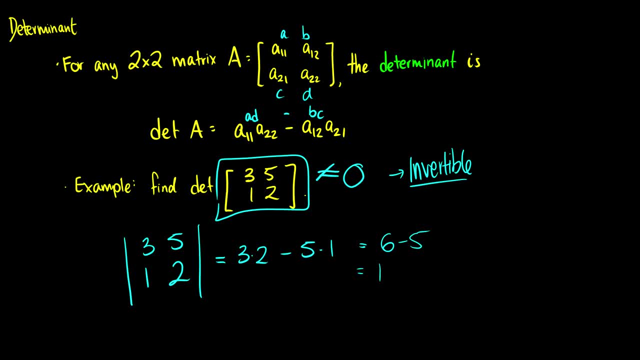 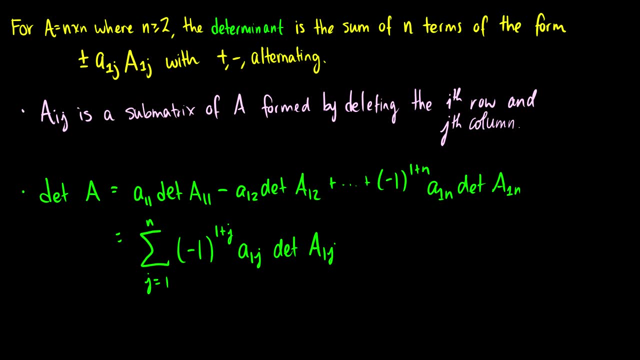 we did show that before. If the determinant is not equal to 0, then the matrix is invertible. OK, so let's go bigger. Let's go to n by n, where n is greater or equal to 2.. So then we say that the determinant is the sum of n terms of the form plus or minus A1j. 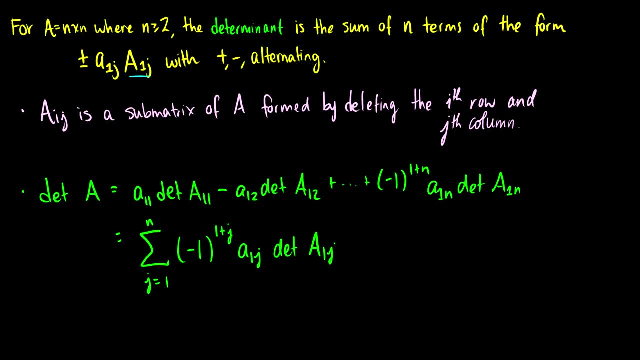 capital A1j, And these pluses and minuses are going to alternate, So first let's talk about what this A1j is. So Aij is the submatrix formed by deleting the i-th row and the j-th column. 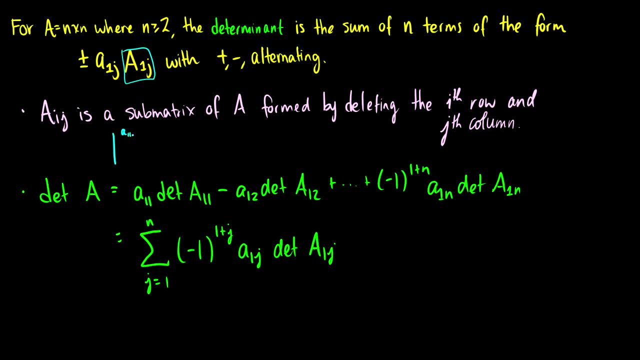 So, for instance, let's say we have A11,, A12, A13.. I'm going to fill in all these entries here. So this would be whoops. that would be 3, 2, and A12, A13.. Submatrix. So that's A. 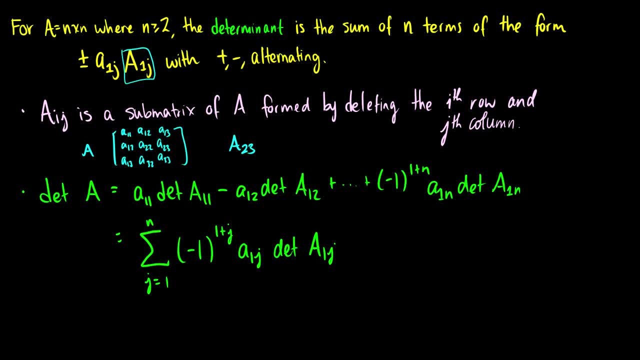 So then let's say A23.. So to form A23, what we do is we remove the A23 from the matrix. So let's say that we remove the A23 from the matrix, So let's say second row, and we remove the third column, So then in our matrix we're left with a11,, a12,, a13,. 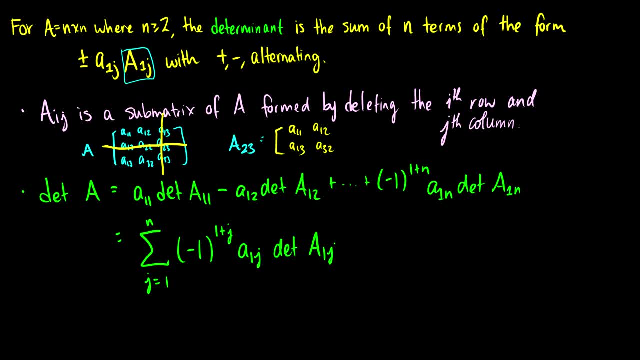 and a32.. So in our final column, our second entry is: well, that's our column that we're getting rid of, so we're never going to get a something. three, in our last column, And we're getting rid of the second row, so we're never going to have a row that starts with the entry two. Okay so, 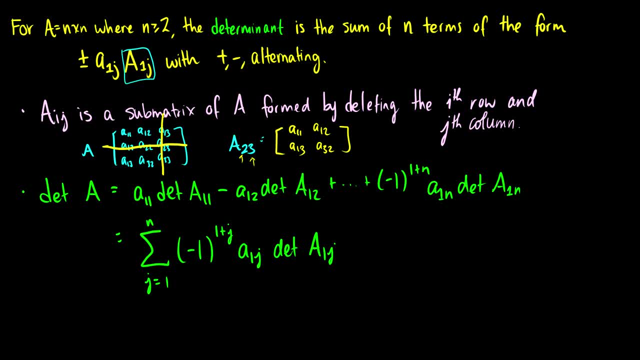 that's how we do things here with our submatrixes. So, with that being said, the full definition of the determinant, if I write it out here, is going to be a11- determinant of a11 minus a12 determinant of a12, and we'll go all the way up to negative one, to the one plus n a1n determinant. 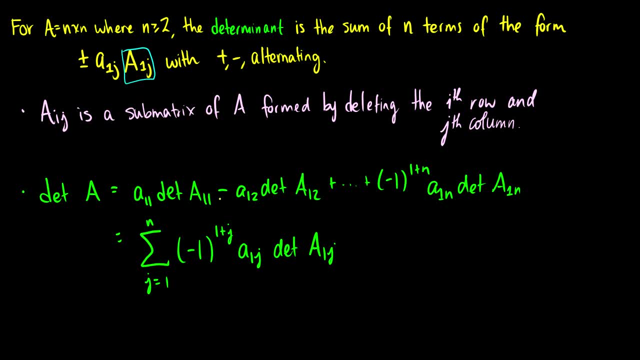 h. So again we have to go plus or minus between all of these. So this sign is going to be dependent on negative one to the power of one plus n. Our first one is positive, which means for every even term. for every second term it has to be negative. Okay, so we can also write this as the 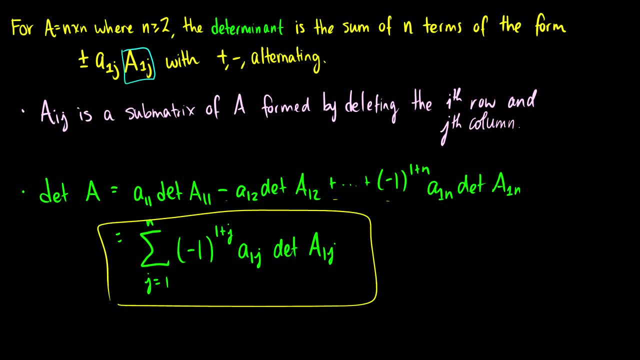 sum. So in proofs you might see the sum being used. Don't be scared of the sum, just remember the general idea of it. So you're taking your terms and then you're going to get the sum. We're going to subtract every other term, Okay. so let's do that. Let's compute the. 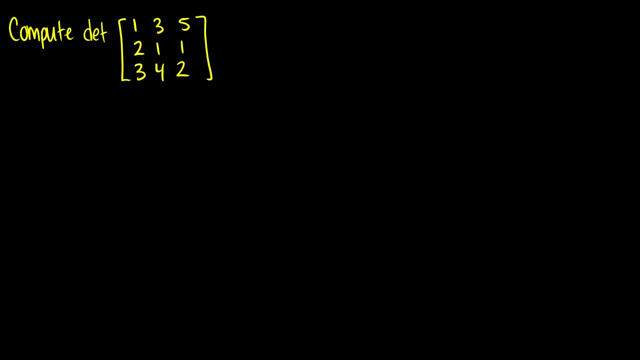 determinant of 135211342.. Okay, so we want to start out, and I'm going to do this very formally here, So I'm going to label everything. So what's the formula for the determinant? So the determinant of a is going to equal a11 times the determinant of capital A. So 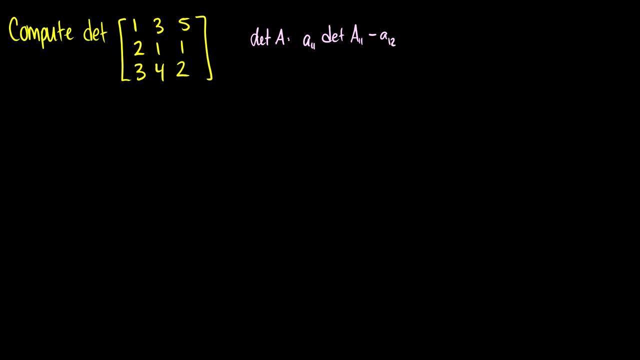 A11 minus A12 times the determinant of capital. A12 plus A13 times the determinant of A13.. So let's start putting in some values here. So the determinant of A is going to be well, A11 is 1 times the determinant of A11.. So this one is done by taking out the first column of A. 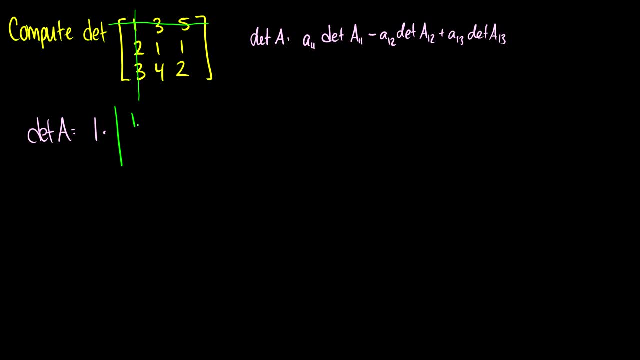 and the first row of A. So then we're going to be left with 1, 1,, 4,, 2.. Okay, so that's A11.. Then we have to subtract A12, which is 3, times the determinant of capital, A12.. So that's taking. 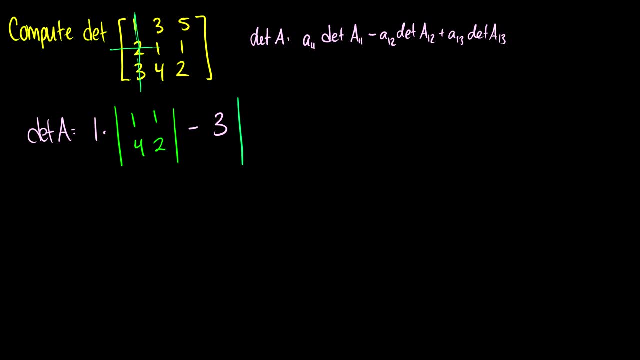 out the first row and the second column. Oh sorry, that would be the first row and the second column, So we're going to be left with 2, 1,, 3,, 2.. And finally, we have to add A13,, which is 5,. 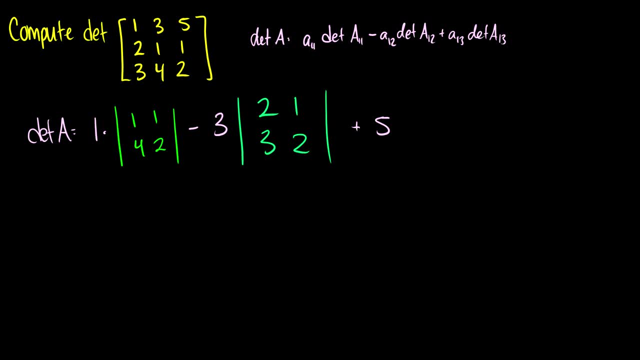 times the determinant of capital A13.. So that's going to take out the first row and the third column. So we're left with 2, 1,, 3, 4.. So at this point we're down to the 2 by 2 case. So we know. 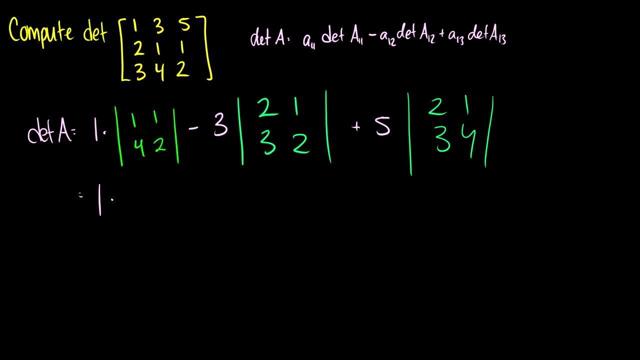 how to take the determinant of that. So we're going to get 1 times. well, remember it's AD minus BC, or the diagonal entries minus the diagonal entries. So it's going to be 1 times 2 minus 1 times 4.. We're going to subtract and the determinant of the second one here is going: 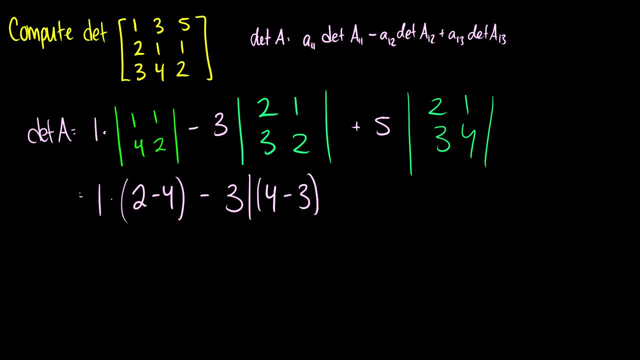 to be 2 times 2 minus 1 times 3.. And we're going to add 5 times the determinant of the third matrix. So this is going to be 2 times 4 minus 1 times 3.. Put these all together, we get negative. 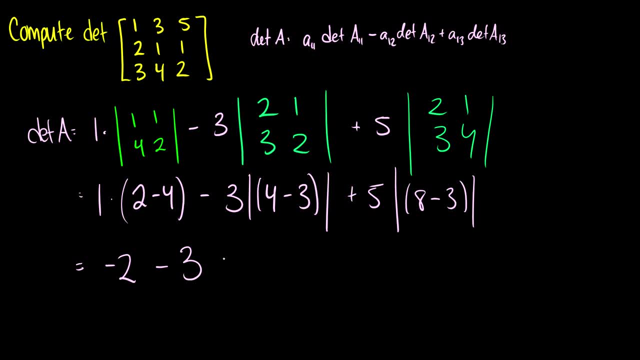 2 minus 3 plus 20.. So our determinant is going to be equal to 20.. Okay, so this is a recursive definition, because we take 3 by 3s, 4 by 4s, 5 by 5s. 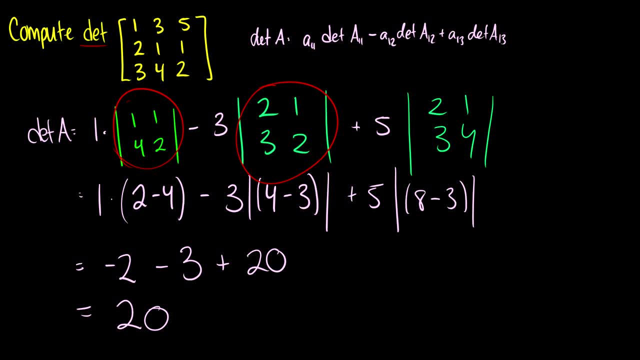 and we reduce them until we get down to 2 by 2s, which we can then solve numerically. So if I ever give you a 4 by 4 determinant, it is going to take quite a bit of time, So I probably won't do that. So let's just do one more example here. 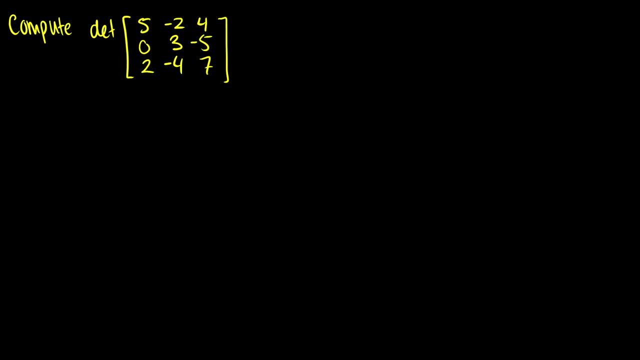 I figure you know, one example probably isn't good enough, So let's do two, And let's do it with some negatives, so that way we can get ourselves confused with the adding and subtraction signs. So I'm not going to do this as formally this time. 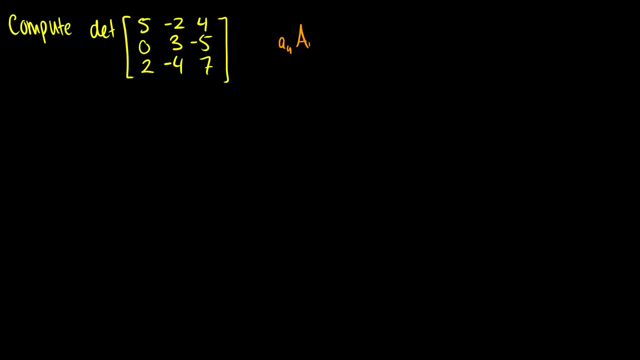 So we're going to say: okay, this is A11, capital A11, minus A12, capital A12, plus A13, capital A13.. I have no reason to write the determinant symbol now, because if I'm using capital A's, 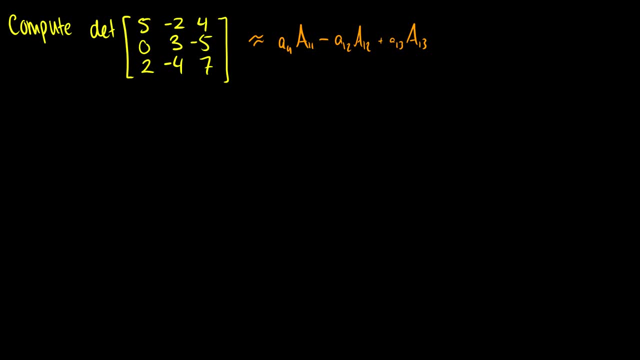 I probably know what I'm doing, So roughly that. So let's start. Well, it's going to be 5 times the submatrix A11.. So at this point I could physically cross these out to help myself. But really what I'm doing is I'm thinking: okay, so here's the 5.. 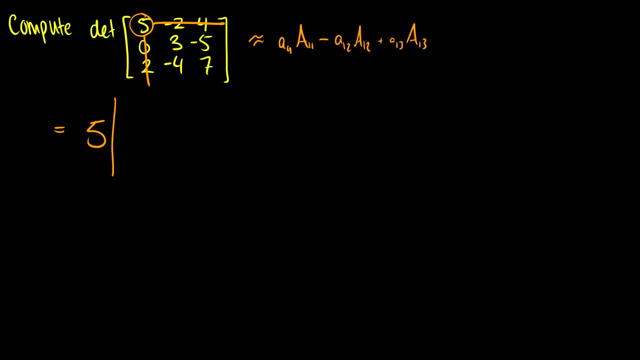 So everything to the right of it. I'm going to ignore everything below it. So that's what I'm thinking in this case. So I'm just going to write the remaining 3, negative 5, negative 4, 7.. 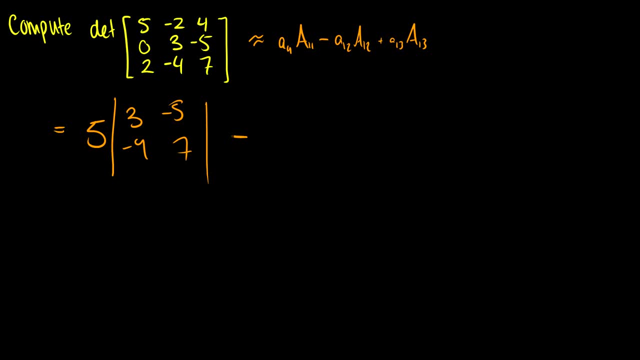 And then we're going to subtract A12, which is negative 2, times the submatrix. So again, I take a look at this 2.. I think, okay, everything below it and everything to the left and right, just ignore it. Okay, so I'll do that. 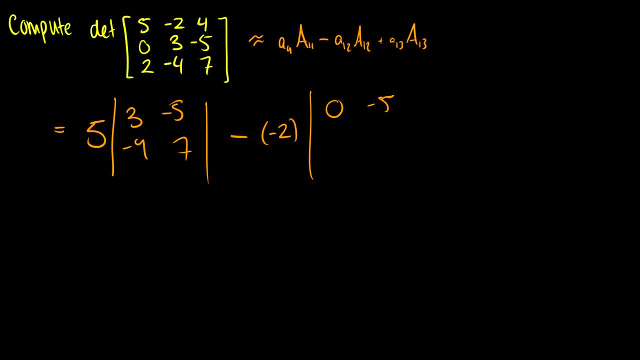 And we're left with 0, negative, 5,, 2, and 7.. I'm going to add A13, which is 4, times, of course, the matrix, ignoring the first row and the third column. so we're left with 0,, 3,, 2.. 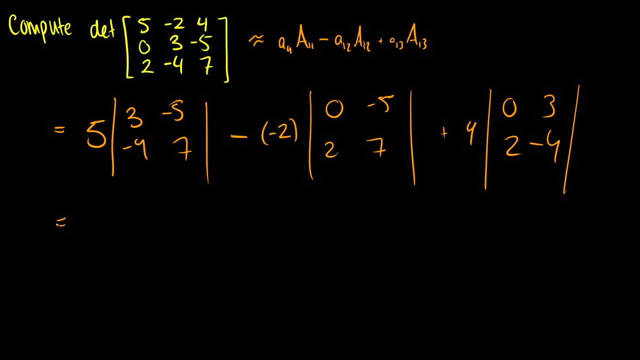 And we're going to add 0,, 3,, 2, negative 4.. Okay, so now these are going to be a little bit more complicated, just with arithmetic. So 5, and here for our determinant, we're going to have 21 minus. 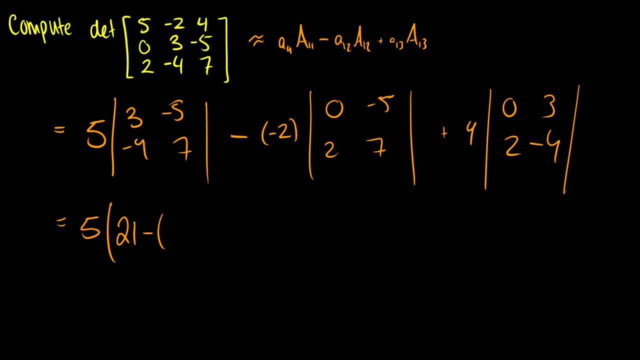 negative 4 times negative 5 is 20.. So 21 minus 20.. We're going to subtract negative 2 times. well, 0 times 7 is 0.. 2 minus 5 is negative 10, so we're going to subtract negative 10.. 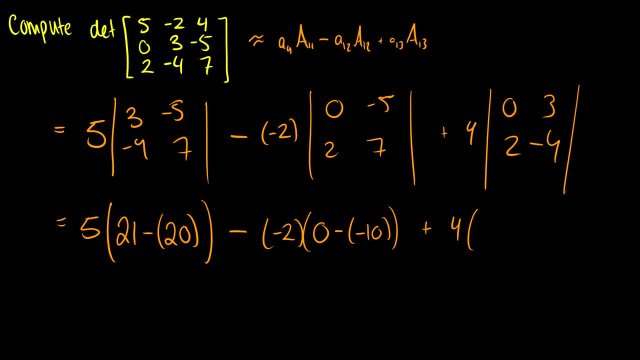 And we're going to add 4 times well, 0 times negative. 4 is 0,. minus 2 times 3 is 6.. Okay, so this is going to be 5 times 1,, which is just equal to 5.. 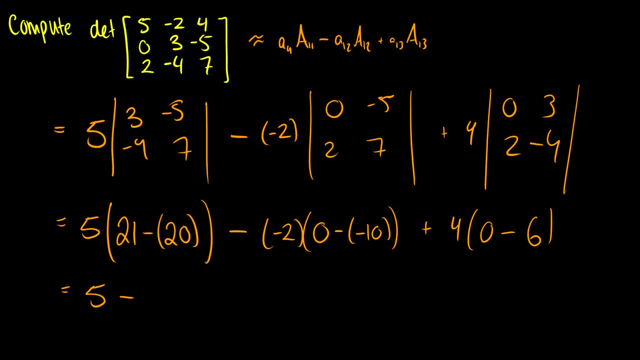 We're then going to subtract okay, so we have negative 2 times 10.. That's negative 20.. So we're going to subtract negative 20, so we're going to add 20.. And then we're going to add 4 times negative 6, which is negative 20.. 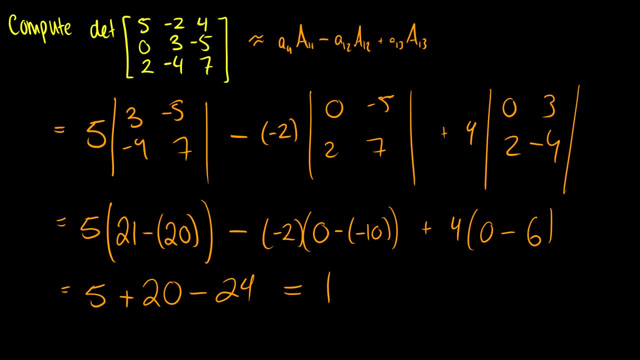 So our determinant is going to be 1.. Okay, so there's a few things you need to watch out for. You need to make sure that your negative signs and positive signs are alternating. So that's why, when I put this in this negative 2, I left it in as is.